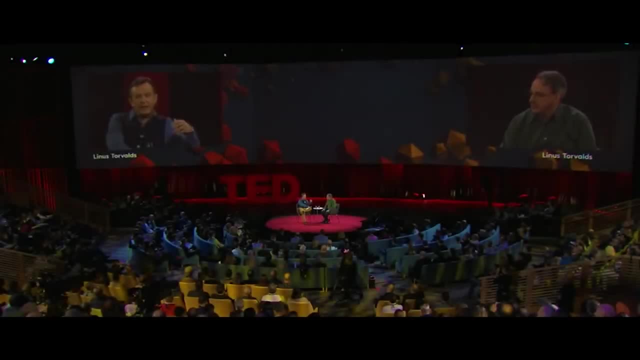 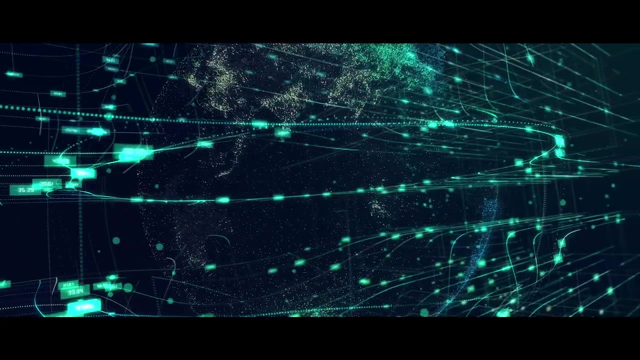 This is such a strange thing. Your software, Linux, is in millions of computers. It probably powers much of the Internet, And I think there are like a billion and a half active Android devices out there. Your software is in every single one of them. 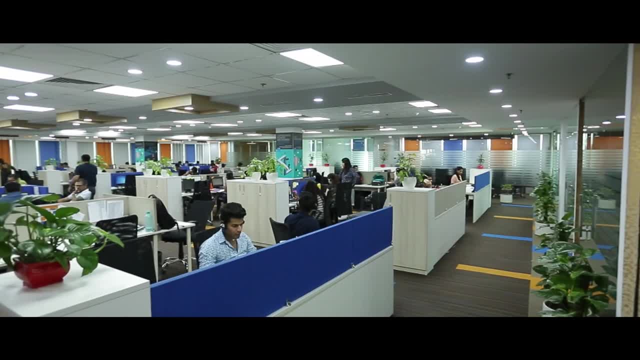 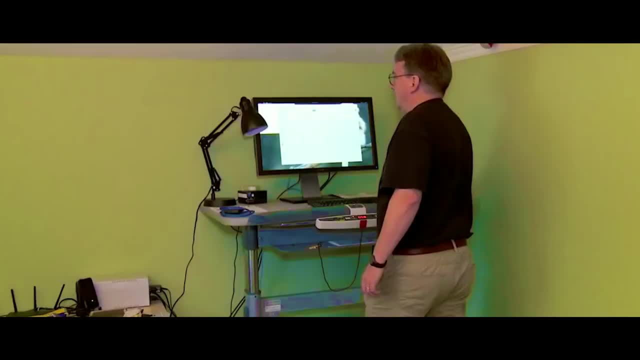 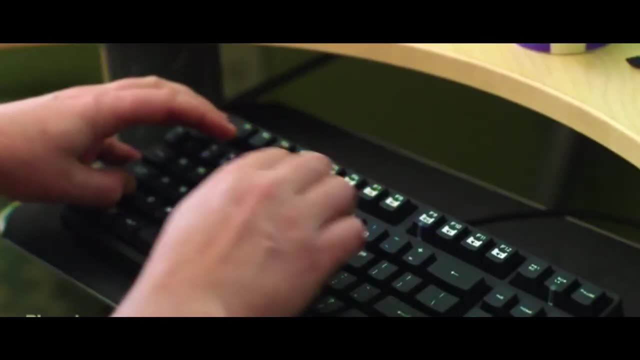 It's kind of amazing. You must have some amazing software headquarters driving all this. That's what I thought, and I was shocked when I saw a picture of it. I mean, this is the Linux world headquarters. Well, I do code for fun, but I want to code for something meaningful. 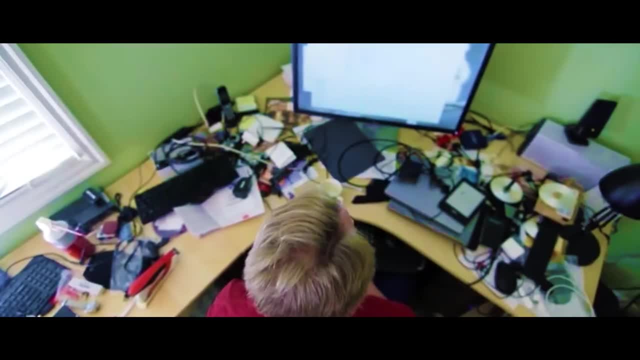 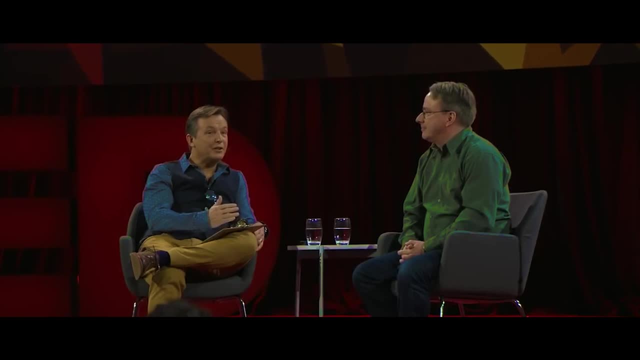 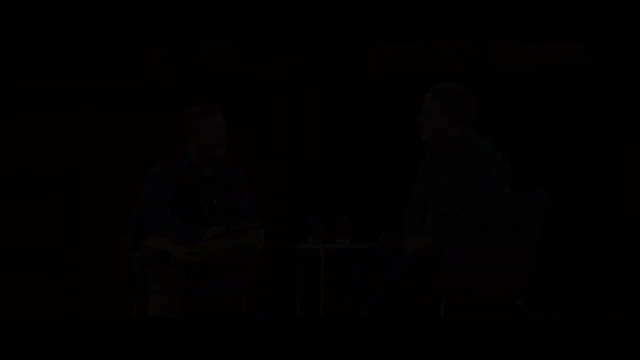 So every single project I've ever done has been something I needed. So really, both Linux and Git kind of arose almost as an unintended consequence of your desire not to have to work with too many people. Absolutely yes, That's amazing, I think everybody 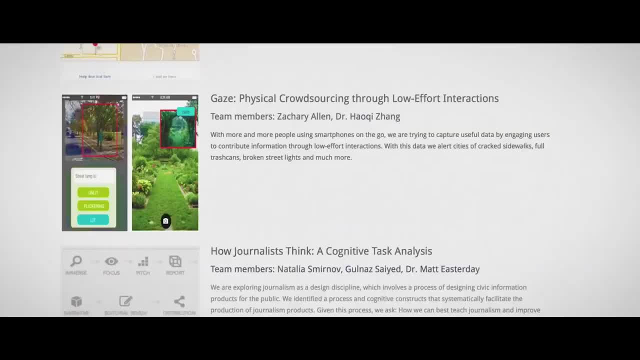 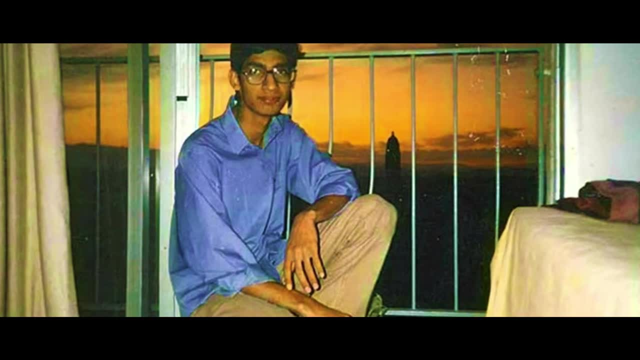 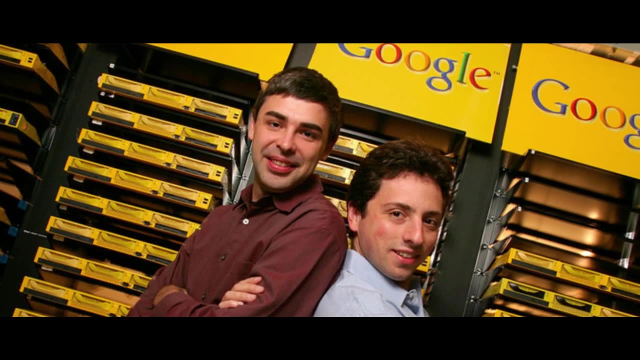 Everybody in this country should learn how to program a computer, Should learn a computer language, because it teaches you how to think. It's the idea that matters. It didn't matter where you come from or what your background is. One revolutionary idea, one brilliant invention can unleash other entrepreneurs to revolutionize industries in ways you could never predict. 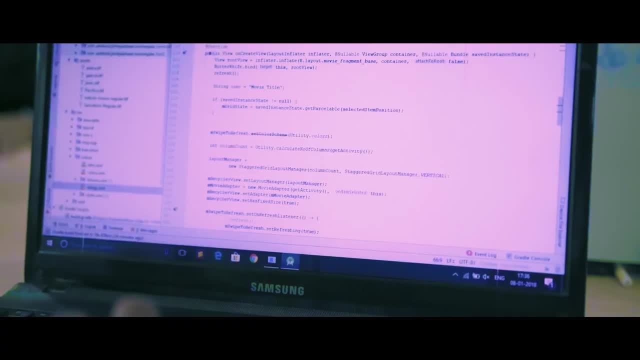 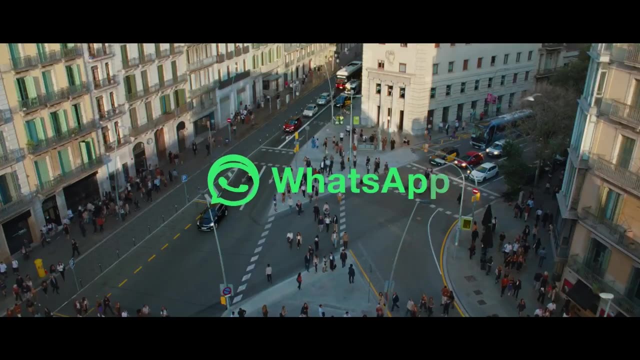 People working anywhere in the world, born anywhere in the world, can create a product and make it available to anyone in the world. There are many applications that wouldn't possibly make it in the world. The most used messaging app in Southeast Asia was built by a young man born in Ukraine who moved to the US. 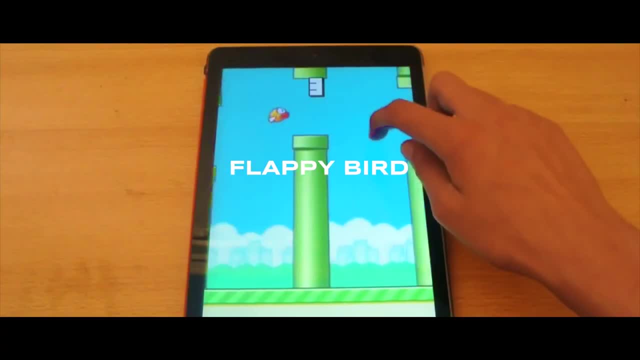 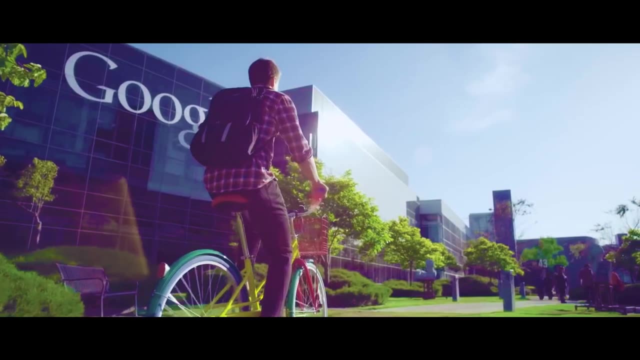 And the three most popular viral games in the US in recent years came from entrepreneurs in Finland, Ireland and Vietnam. You're the ones building the next Google, the next Spotify, the next Tesla, the next what we don't even know. 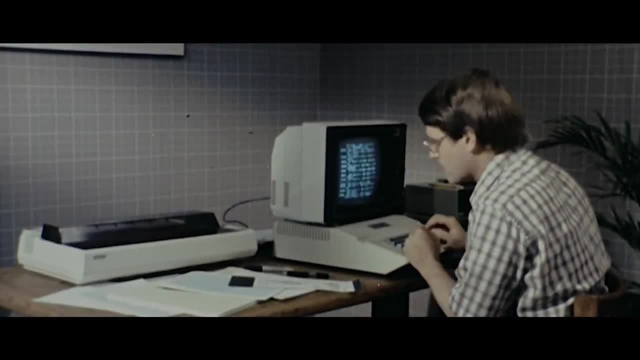 But what I know is that someone in this room will will build it". Computer science is by far the greatest And the word of the century is still spilling to everyone. the wordmaker, the like TheUnis are the world. It's gone. 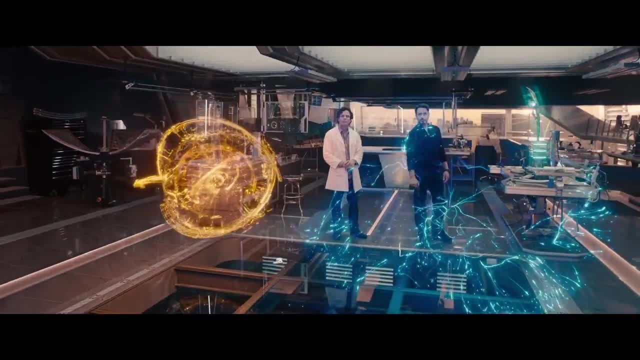 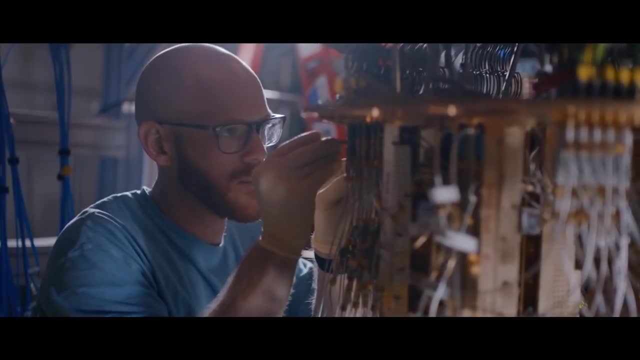 But I don't know how we can beWAI. There is no law for all features closest thing to magic, and it's certain that the world wouldn't be where it is right now without the existence of this magnificent branch of science. and this branch of science is growing so fast that it's difficult for even good.